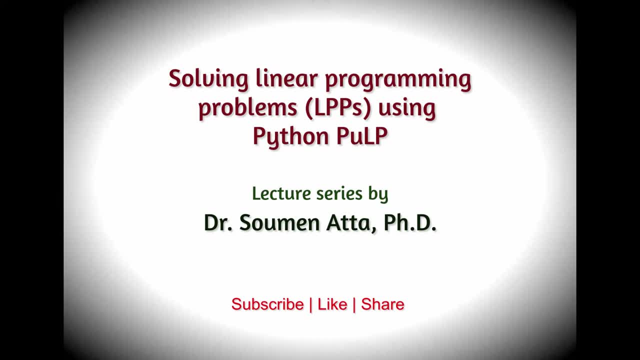 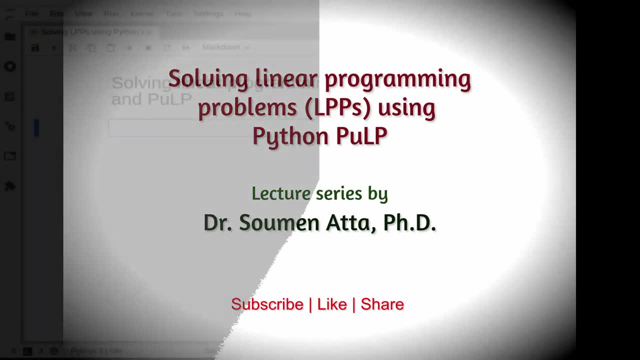 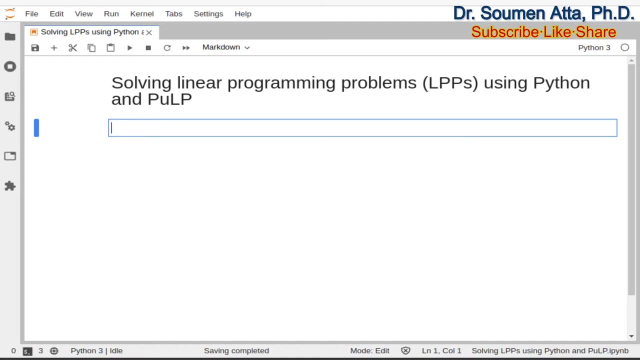 Dear students, in this tutorial we will learn how to solve linear programming problems- LPPs- using Python and pulp. At first we will learn how to install pulp. If pulp is already not installed in your system, then you can use the following commands to install it: 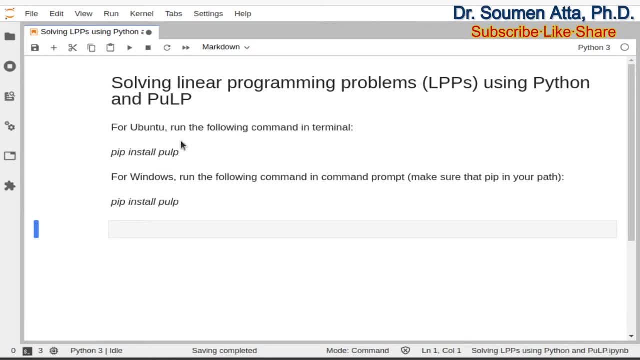 Here are the two commands. Here I am using Ubuntu 20.04 LTS operating system. You can install pulp using pip command in Ubuntu. You can also use the pip command to install pulp in windows. In case of windows, make sure that pip is in your path Here we will solve. 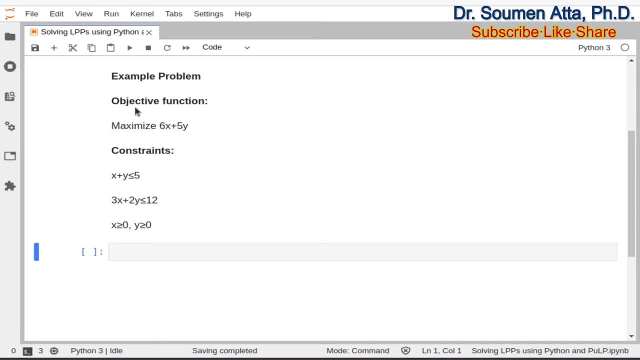 this LPP using pulp. Here you can see the objective function is maximize 6x plus 5y and we have setup constraints: x plus y less equal to 5. 3x plus 2, y less equal to 12.. We have here 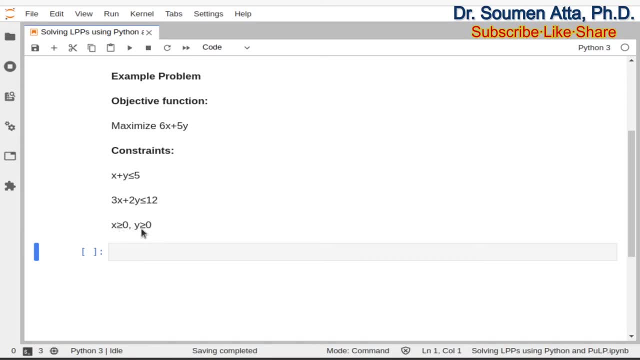 also two non-negativity constraints: x greater equal to 0 and y greater equal to 0.. In this tutorial, we will learn how to solve this LPP using pulp. At first we need to import the required brackets, We need to import pulp using the command, and then we need to instantiate a problem class. 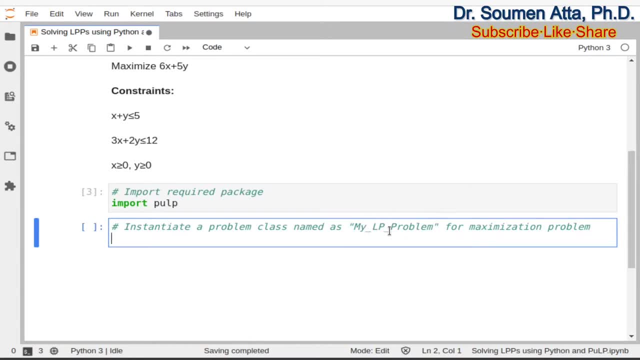 named as mylpproblem, my underscore lp underscore problem for maximization problem, and the command is like this: mylpproblem equal to pulp dot lp problem, and within the round brackets you need to mention my underscore lp underscore problem and here we are solving a maximization. 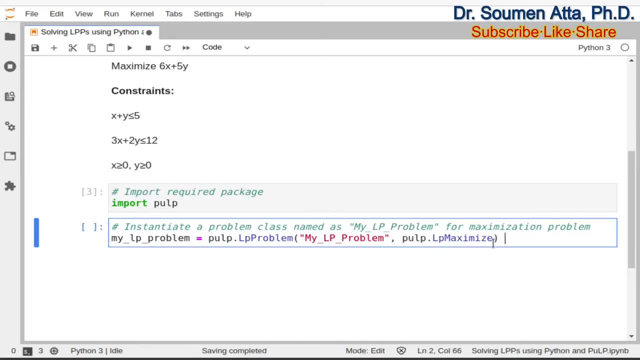 problem. So we need to mention here pulp dot, lp- maximize. This command will instantiate a problem class named as my underscore lp underscore problem for maximization problem. Now I will show you how to define the decision variables. For our example problem we have two decision variables, x and y. 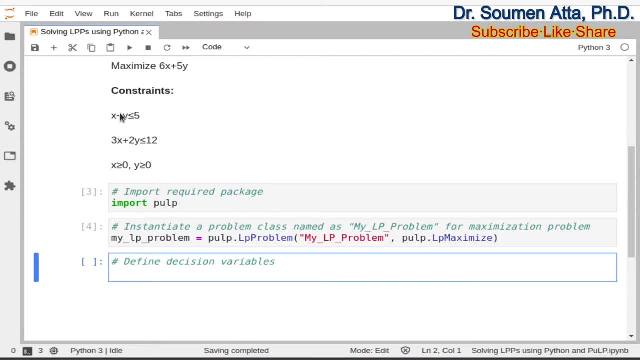 Now we will define the decision variables. For the example problem we have two decision variables, x and y. The decision variable x can be defined like this: x equal to pulp, dot, lp variable, And within the round brackets you need to mention the name of the variable, that is, x. 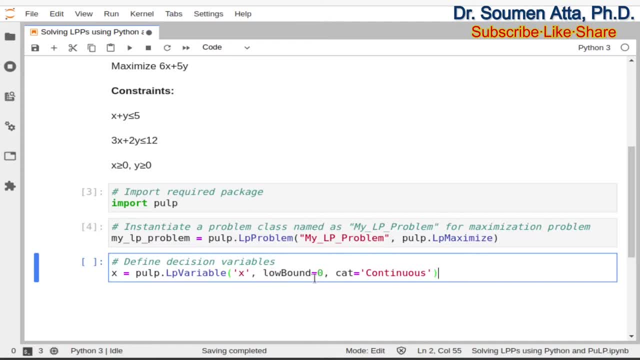 You need to mention the lower bound. here the lower bound is zero, as you can see that x greater equal to zero. and you also need to mention the category of the variable, and here it is a continuous variable, since we are considering LPP. therefore, the decision variable is a continuous. 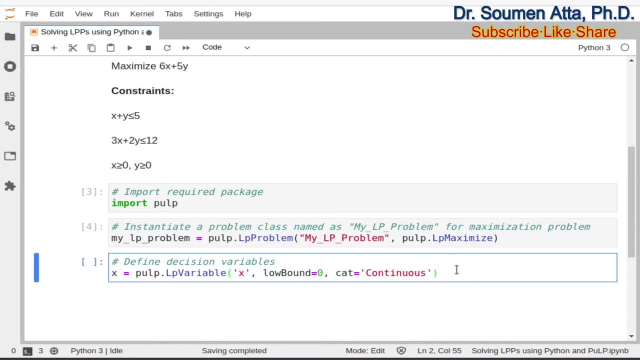 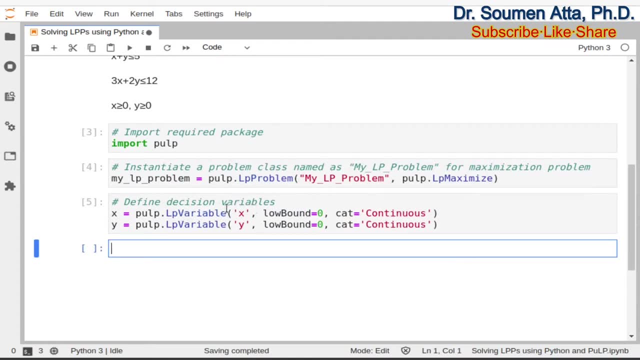 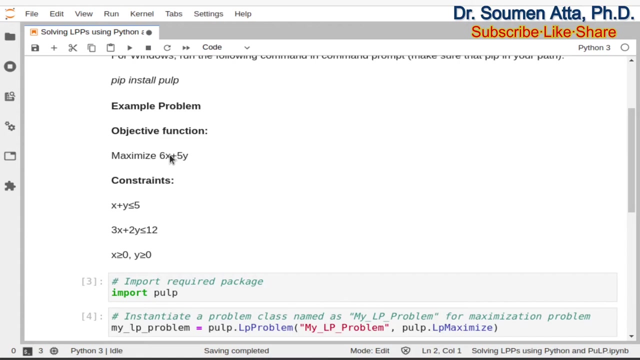 variable. Similarly you can also define the decision variable y like this: Now we have successfully defined the two decision variables of the given problem and the decision variables are x and y. Now I will show you how to define the objective function. So in the given example problem we have the objective function like this: maximize six. 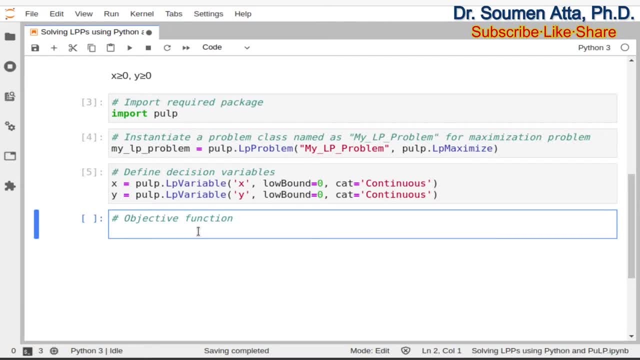 x plus five y, and this can be defined using the pulp command like this. So my underscore lp, underscore problem plus equal to six x plus five y. This is the name of the objective function that we have given. in general, the objective function in LPP is denoted by z. 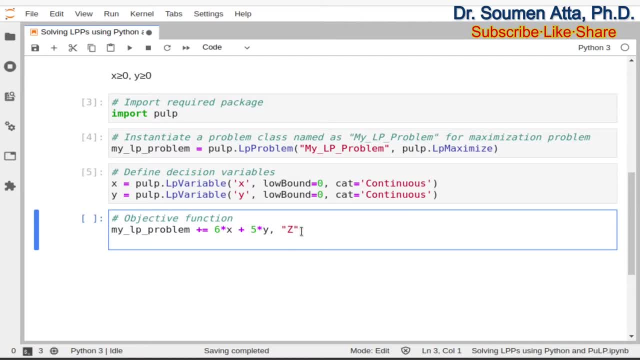 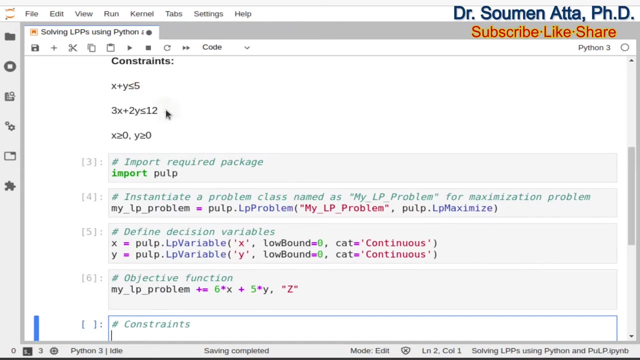 So that's why here I have used z. you can use your own name also. So this command will define the objective function. Now I will show you how to define the two constraints here. the two constants are x plus y less equal to five, and three x plus two y less equal to twelve. 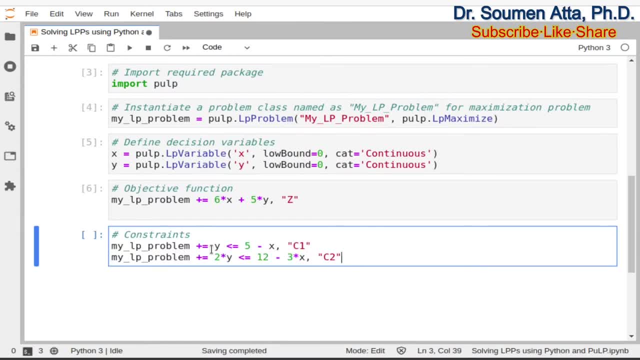 The commands are as follows: my underscore lp underscore problem: plus equal to y, less equal to five minus x. Actually, here in pulp you need to write down the constants in the form y equal to f of x. So here you can see that only y is kept at the left hand side. 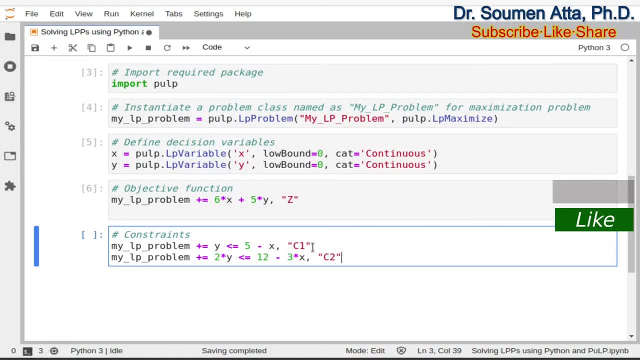 So y less equal to five minus x and c one. again it denotes the name of the constant. So it's the first constant. that's why I have given the name c one. in the similar fashion, the second constant has the name c two, and here you can also see: 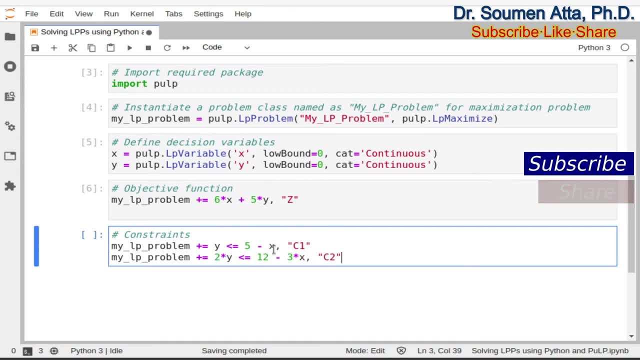 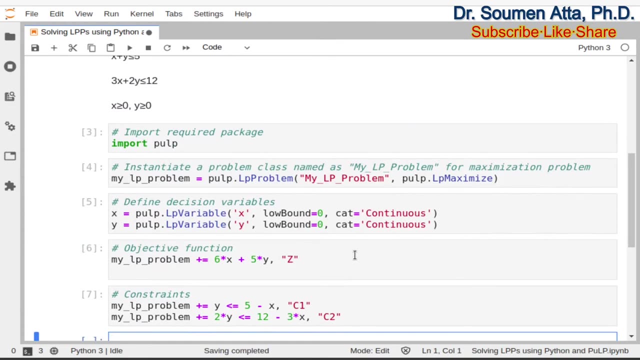 that two y less equal to twelve minus three x. So all the x terms and the constant terms are on the right hand side and the y terms are on the left hand side. So these two commands will define the constants in pulp. And here note that you don't need to define the non negativity constraints. that means 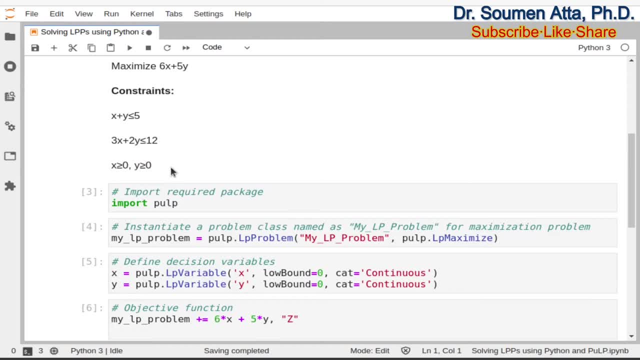 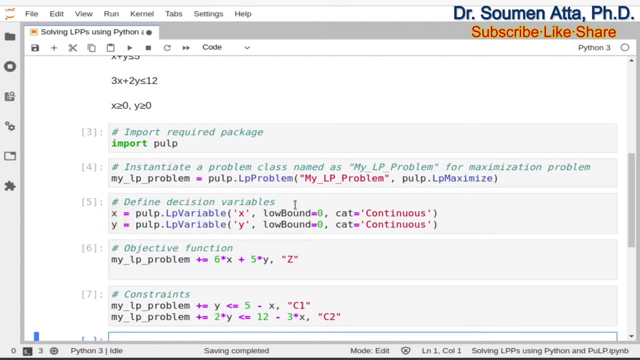 x greater equal to zero And y greater equal to zero, Because it is already defined when you have defined the decision variable x and y. So here you can see that the lower bounds for both x and y are zero and it is a continuous variable. 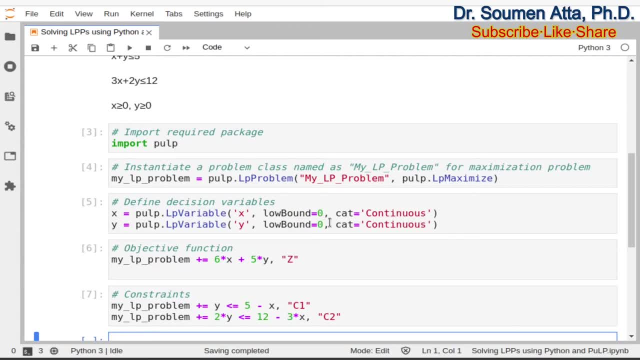 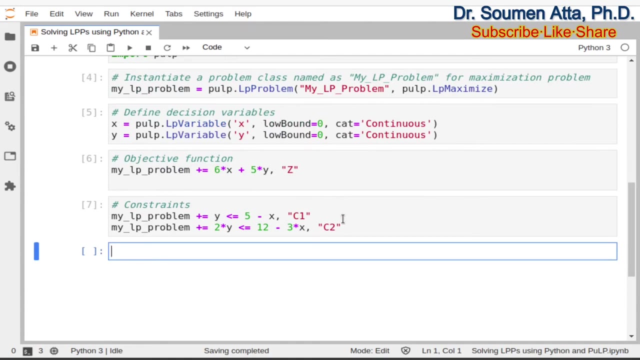 Both these variables are continuous. therefore, by definition of the decision variables x and y- this non negativity constraints- x greater equal to zero and y greater equal to zero- is covered. So now you have created your pulp model for the given LPP and if you want to print your 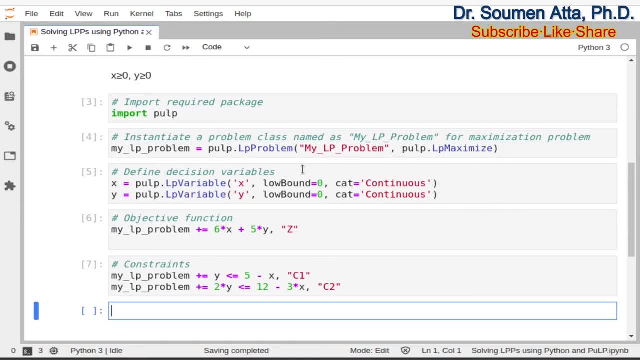 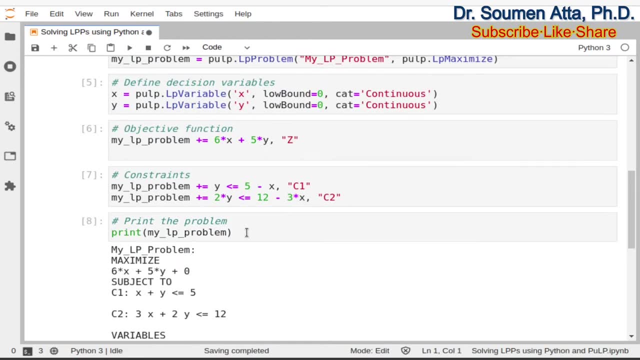 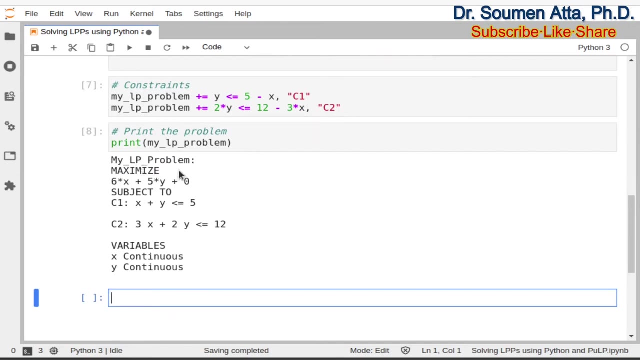 problem. that can also be done. for that you need to write down a command like this: print my underscore- lp underscore- problem. So this will print the problem that you have modeled. So here you have created an instance of the problem class named as my underscore lp underscore. 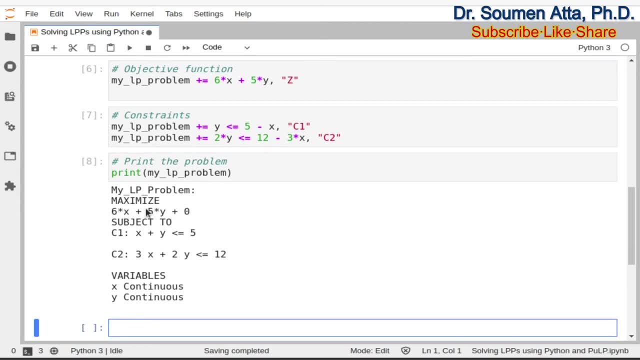 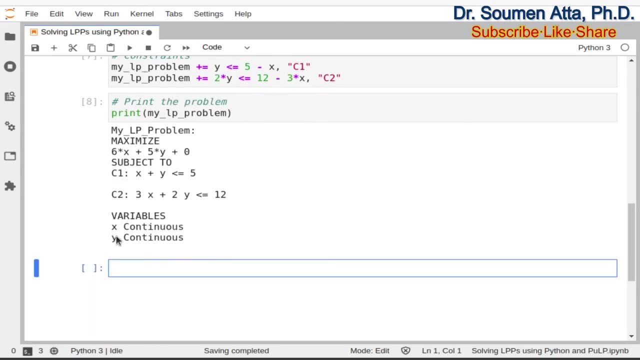 problem. This is a maximization problem, and here you can see the objective function and here you can see the two constraints and here you can see the list of decision variables x and y, and in this case both are continuous. Now to solve the ABHOP LP model using pulp, you just need to write down the command like: 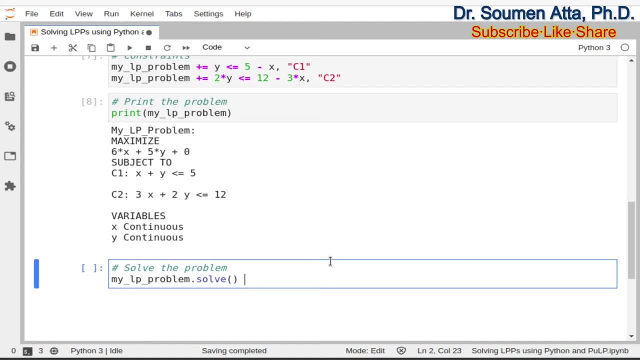 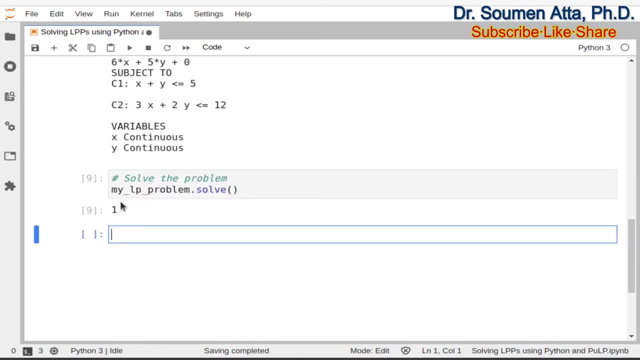 this my underscore, lp. underscore problem dot solve, and this will solve the given LP. As you can see, the output is one That means the problem has been successfully solved. Now, if you want to know the status of the problem that you have just solved, you can. 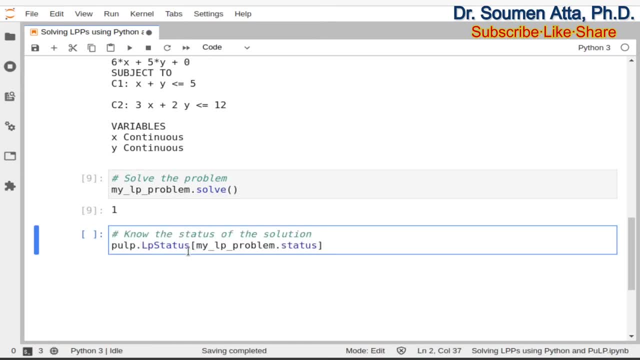 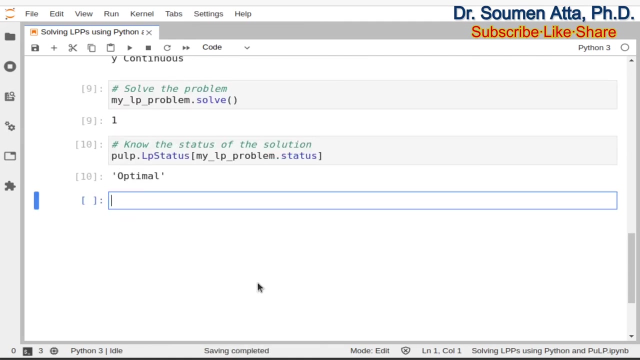 write down the command like this: pulp, dot, lp status and within the square brackets you need to mention my underscore lp, underscore problem, dot status and here, as you can see, it returns optimal. That means the given problem has been solved optimally using pulp. You can also print the value of the decision variables in the optimal solution for that. 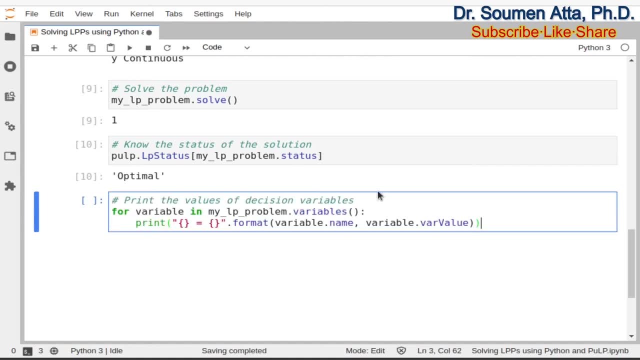 you need to write down the command like this, and this command will print the values of the decision variables in the optimal solution Here. basically, using the for loop, we iterate over all the decision variables and then, using this print statement, we are printing the value of the corresponding decision variable in.